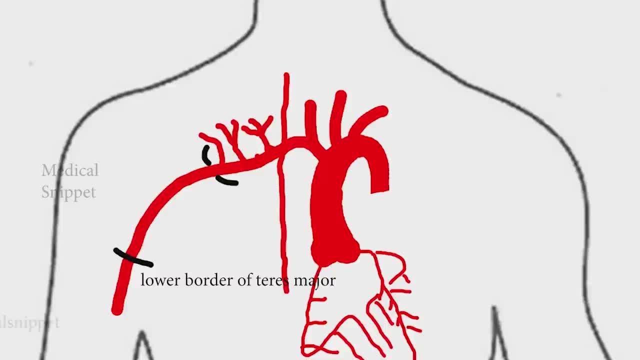 It is divided into three parts by pectoralis minor muscle. The first part gives rise to one branch called superior thoracic artery. The second part gives rise to two branches: thoracoacromian artery and lateral thoracic artery. Thoracoacromian artery splits into four branches: pectoral, acromial, clavicular and deltoid. 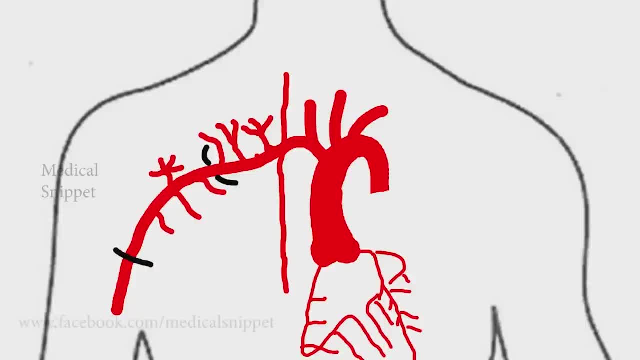 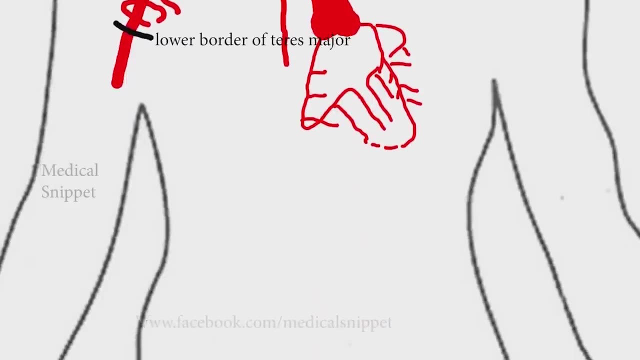 The third part of axillary artery gives rise to three branches. The third part gives rise to two branches: subcapular artery, posterior humeral circumflex artery and anterior humeral circumflex artery. The axillary artery continues as brachial artery from the lower border of teres major muscle. 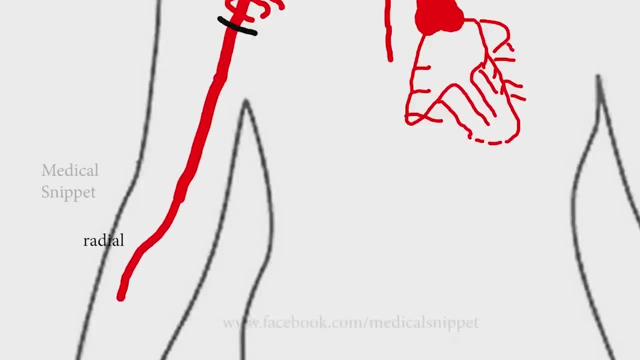 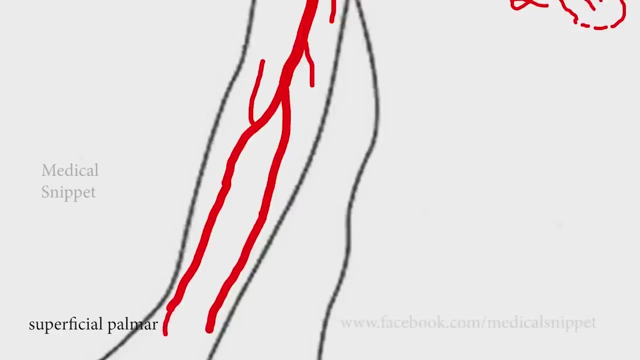 The brachial artery terminates into radial and ulnar arteries. It gives rise to profunda brachii artery, superior and inferior ulnar arteries. The ulnar artery is divided into two branches: ulnar collateral arteries. The radial artery gives rise to radial recurrent artery and superficial palmar branch. 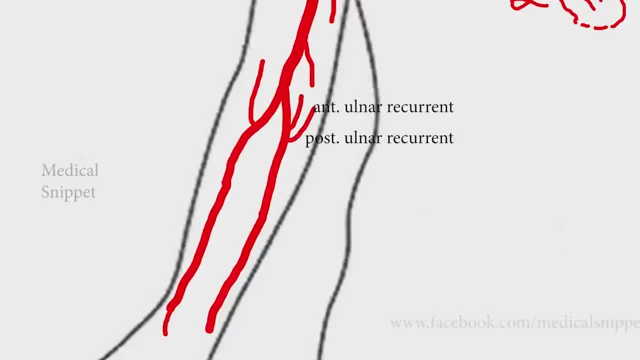 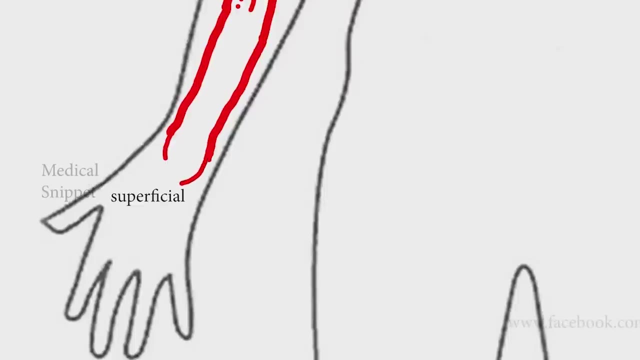 The ulnar artery gives rise to anterior and posterior ulnar recurrent arteries. common interosseous artery, which gives rise to the anterior, posterior and recurrent interosseous arteries. The ulna artery at the wrist divides into superficial and deep branch. 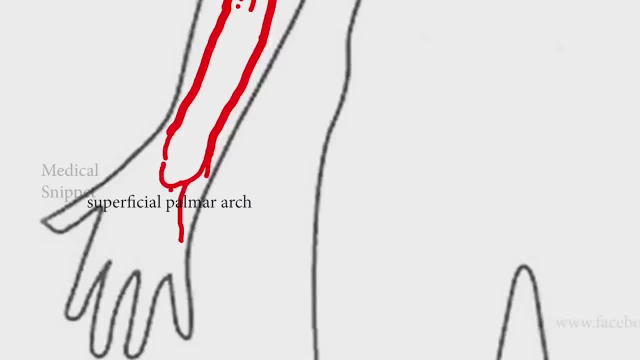 The superficial branch forms the superficial palmar arch which gives rise to four common digital palmar arteries, which in turn gives rise to proper palmar digital arteries. The radial artery continues as deep palmar arch and anastomosis with deep branch of ulna artery. 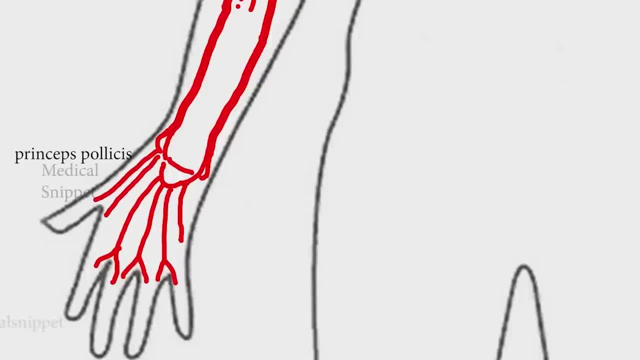 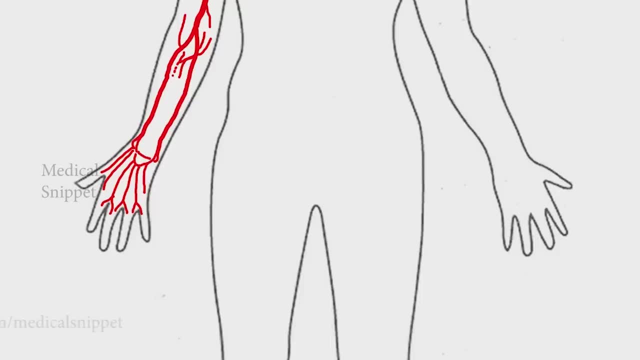 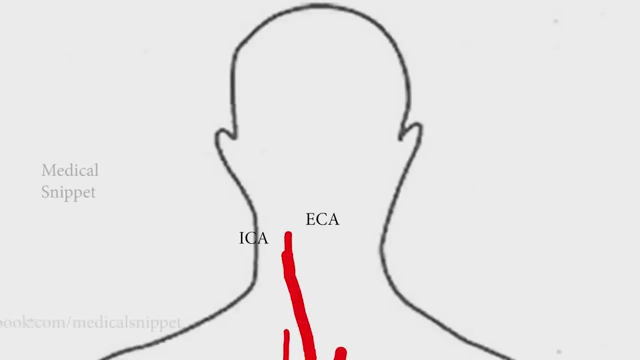 The deep palmar arch gives rise to princeps pollicis artery and radialis indicis artery. Let's see the arterial tree of head and neck. The common carotid artery divides into external and internal carotid arteries. The external carotid artery terminates into superficial, temporal and maxillary arteries. 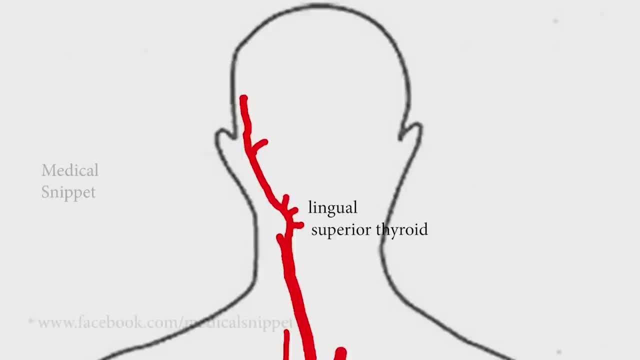 The anterior branches are superior thyroid artery, lingual artery and facial artery. The medial or deep branch is ascending pharyngeal artery and the two posterior branches are occipital and posterior auricular arteries. The internal carotid artery has no branches in the cervical part. 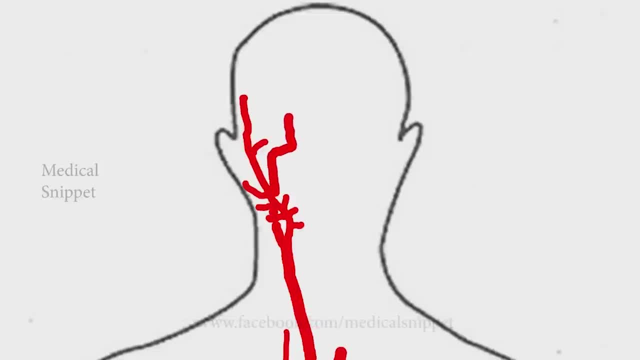 The petros cavernous and cerebral part gives rises to many branches. the important ones are discussed here. The internal carotid artery divides to form the middle cerebral artery and anterior cerebral artery. It also gives rise to posterior communicating artery, the ophthalmic artery and anterior choroidal artery. 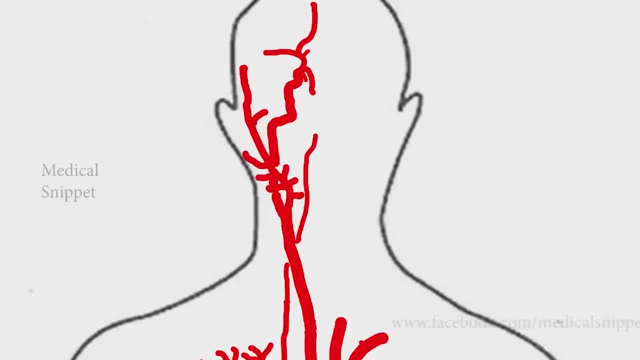 Inside the skull, the two vertebral arteries join to form the basilar artery at the base of the pons. The basilar artery is the main blood supply to the brainstem and connects to the circle of Willis to potentially supply the rest of the brain if there is compromise to one of the carotids. 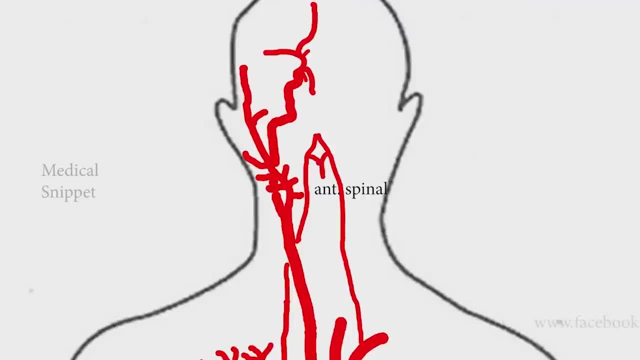 Vertebral artery gives rise to the anterior spinal artery. The basilar artery gives rise to anterior inferior cerebellar artery, superior cerebellar artery and divides into posterior cerebral arteries. It also gives paramedian pontine branches. Let's now complete the circle of Willis. 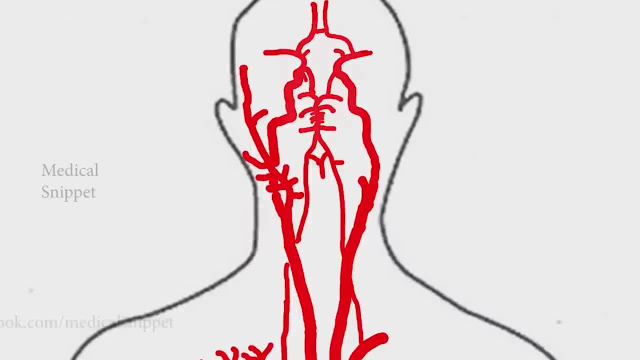 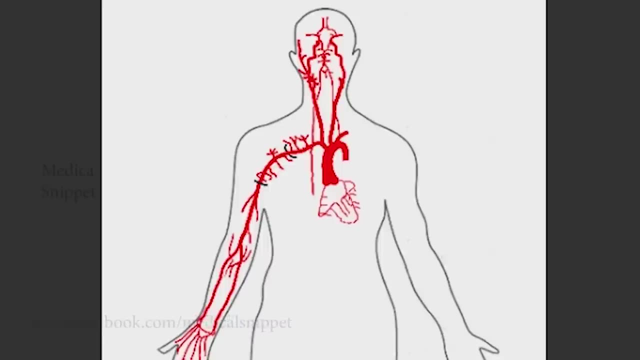 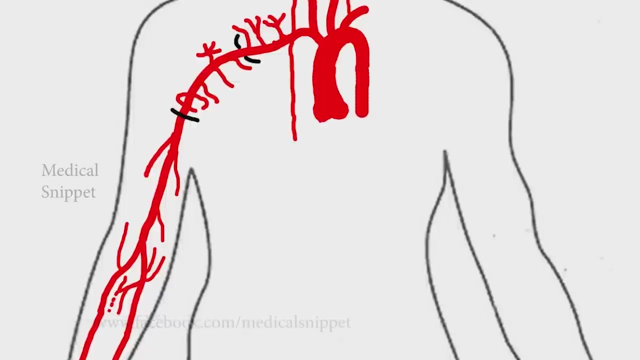 Let's see the branches of descending thoracic aorta. The coronary arteries are temporarily hidden to visualize the descending thoracic aorta. The descending aorta starts at the level of the fourth thoracic vertebral body as the continuation of the aortic arch. 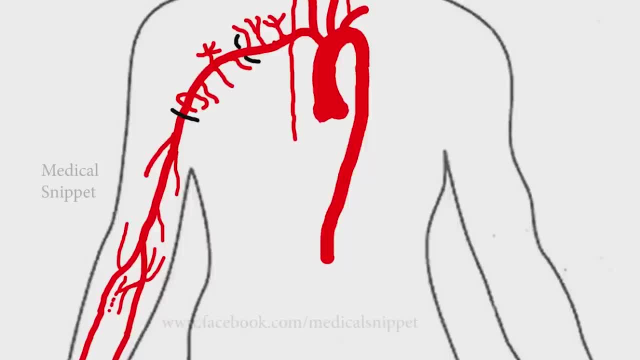 It exits the thorax by continuing as the abdominal aorta. as it crosses the aortic hiatus in the diaphragm at the level of the twelfth thoracic vertebra, It gives rise to nine pairs of posterior intercostal arteries of third to eleventh intercostal spaces. 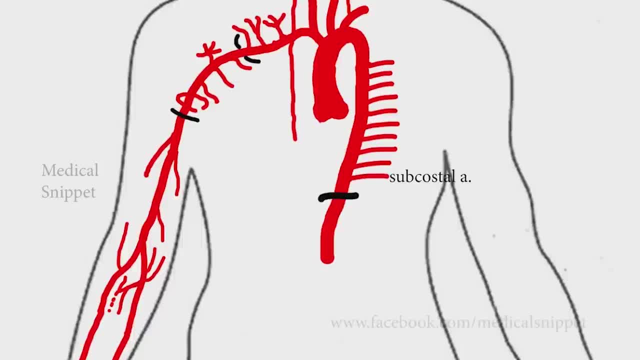 It also gives a pair of subcostal artery and a pair of superior phrenic artery. The first and second intercostal arteries arise from the superior intercostal artery, which is a branch of costocervical trunk of subclavian artery. 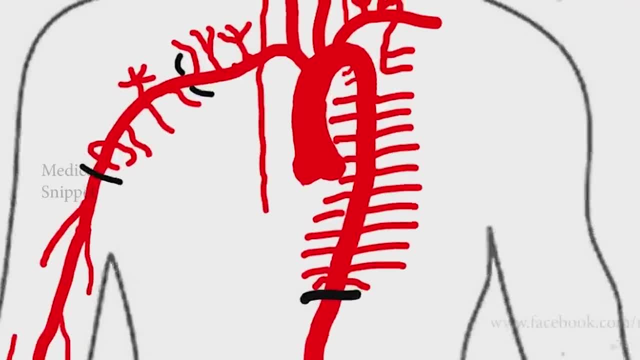 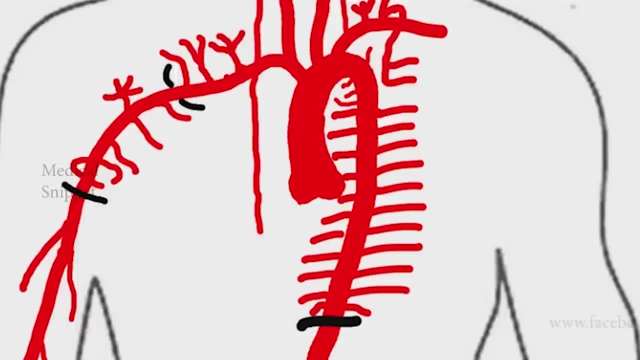 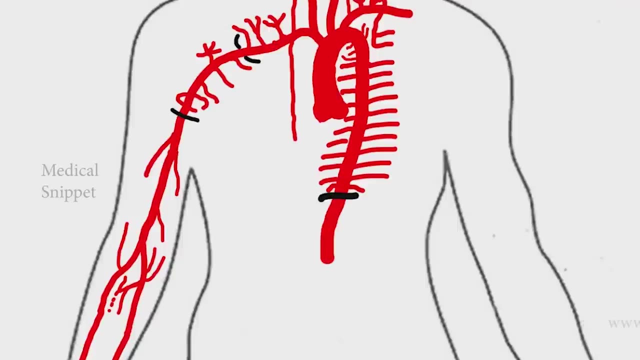 The other branches of descending thoracic aorta are esophageal, mediastinal and bronchial arteries. There are two bronchial arteries on the left and one on the right. Let's see the abdominal aortic branches. Abdominal aorta is continuation of descending thoracic aorta from the aortic hiatus. 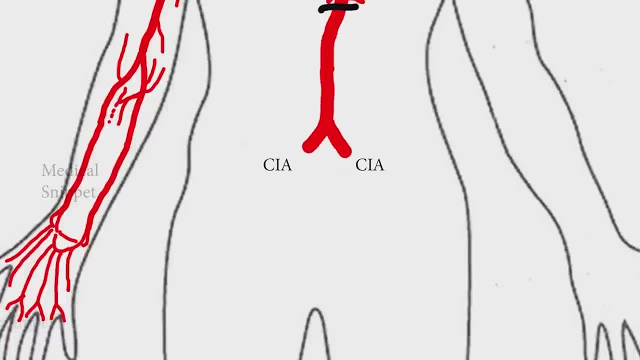 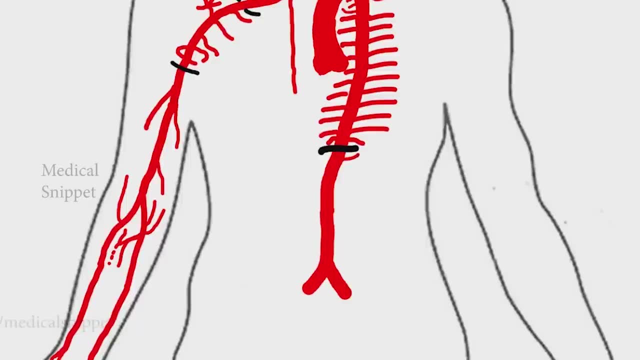 It extends till the bifurcation into common iliac arteries. First we will see the five paired lateral abdominal wall branches: inferior phrenic artery and four lumbar arteries. Next we'll see the three paired lateral visceral branches middle suprarenal artery, renal artery and gonadal artery. 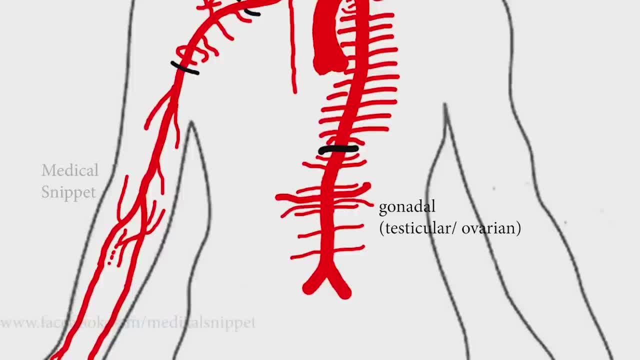 We'll see the three paired lateral venous arteries: testicular arteries in male and ovarian artery in females. The inferior phrenic artery gives rise to superior suprarenal artery and renal artery gives rise to inferior suprarenal arteries. 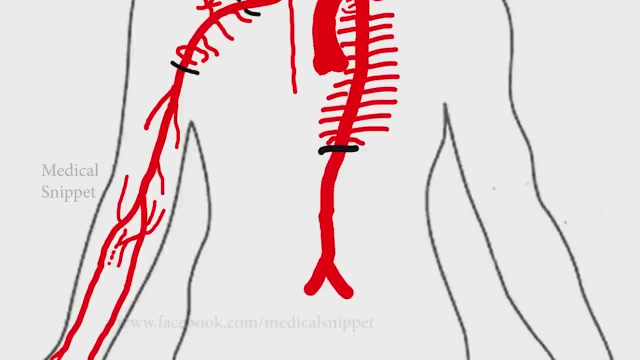 We'll hide the above branches to see the three. three single anterior visceral branches: celiac trunk, superior and inferior mesenteric arteries. Celiac trunk arises at the level of 12th thoracic vertebra. The celiac artery supplies blood to the liver, stomach, abdominal esophagus, spleen and the superior half of both the duodenum and the pancreas. 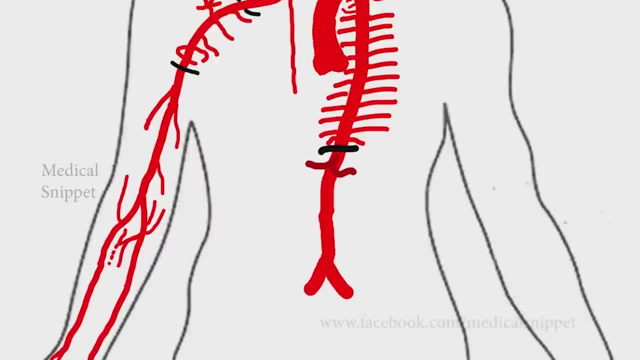 These structures correspond to the embryonic foregut. It divides into common hepatic, splenic and left gastric arteries. Left gastric artery gives gastric and esophageal branches. Splenic artery gives pancreatic, splenic, short gastric and left gastroepiploic arteries. 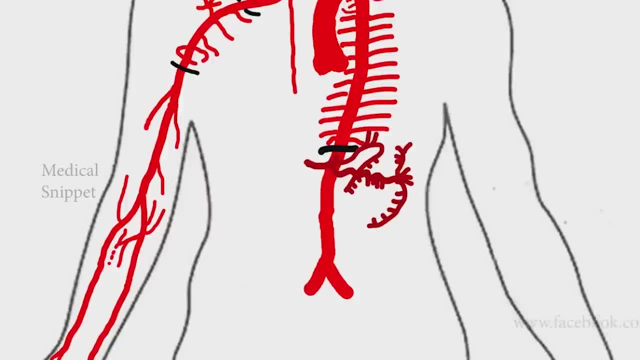 Common hepatic artery branches into proper hepatic artery, gastroduodenal and right gastric arteries. Proper hepatic artery divides into left and right hepatic arteries. Right hepatic artery gives cystic artery. Gastroduodenal artery divides into superior pancreaticoduodenal artery and right gastroepiploic artery. 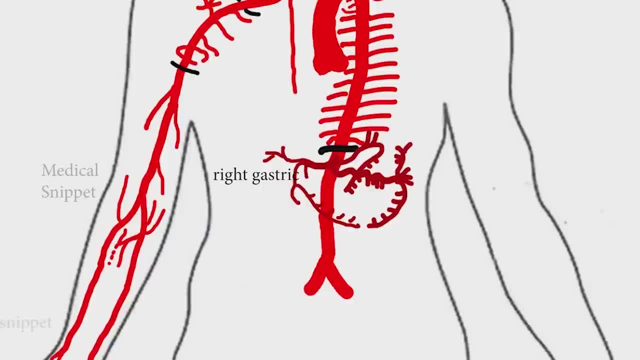 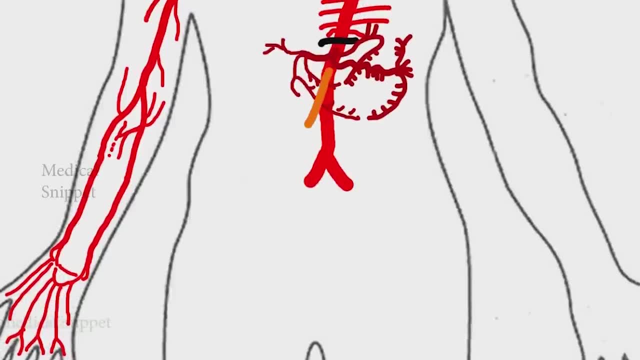 Right gastric artery runs along the lesser curvature of the stomach. Superior mesenteric artery arises at the level of first lumbar vertebra. It supplies the intestine from the lower part of the duodenum through two-thirds of the transverse colon as well as the pancreas. 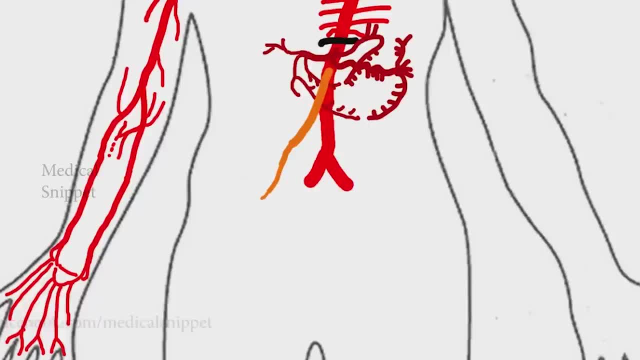 These structures corresponds to the embryonic midgut. It gives rise to inferior pancreaticoduodenal artery, jejunal arteries, ileal arteries, iliocolic arteries, right colic and middle colic arteries. Iliocolic artery gives rise to anterior and posterior cecal arteries. 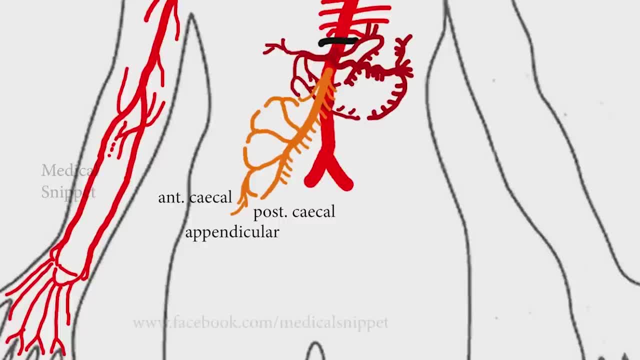 Appendicular branch arises from posterior cecal artery. Inferior mesenteric artery arises at the level of third lumbar vertebra. The territory of distribution of the IMA is equivalent to the embryonic hindgut, That is, it supplies the large intestine from splenic flexure to the upper part of the rectum, which includes the descending colon and the sigmoid colon. 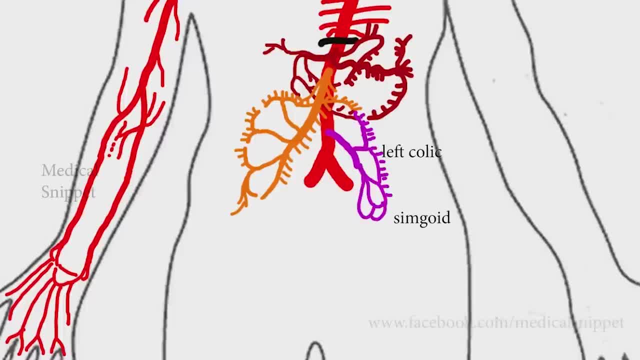 It gives rise to left colic artery sigmoid arteries and it continues as superior rectal artery. The median sacral artery is a small single posterior branch of the distal abdominal aorta. The common iliac artery divides into external and internal iliac arteries. 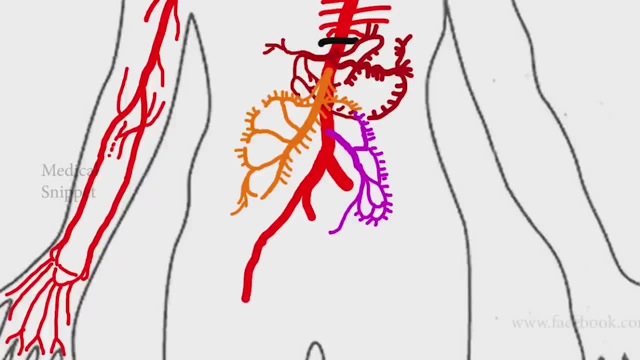 The external iliac artery passes beneath the inguinal ligament and becomes the common femoral artery. External iliac artery gives rise to inferior egogastric and deep circumflex iliac arteries. These vessels supply blood to the muscles and skin in the lower abdominal wall. 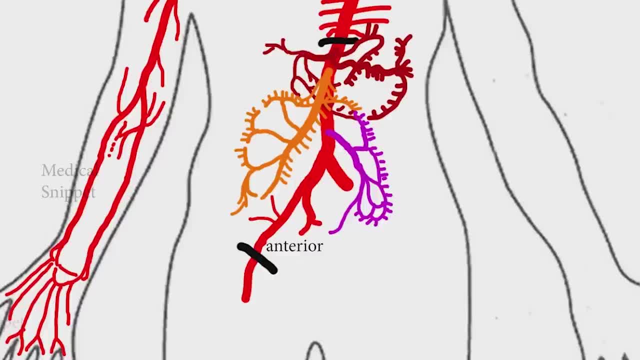 Internal iliac artery divides into anterior and posterior division. Posterior division gives rise to iliolumbar artery, lateral sacral artery and superior gluteal artery. Anterior division gives rise to umbilical artery, and superior vesicular artery arises from it. 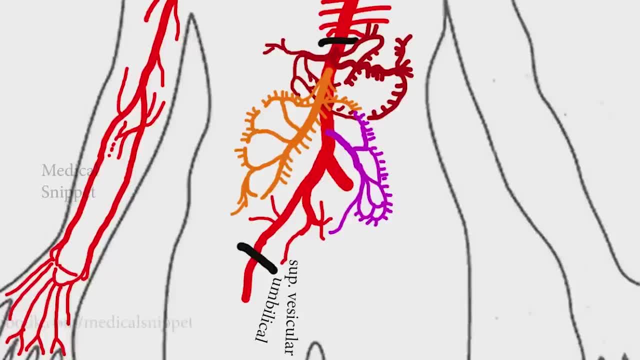 In some people superior vesicular artery arises as a separate branch. other branches of anterior division are: obturator artery, inferior vesicular artery in male or vaginal artery in female, middle rectal artery, internal pudental artery and inferior gluteal artery. 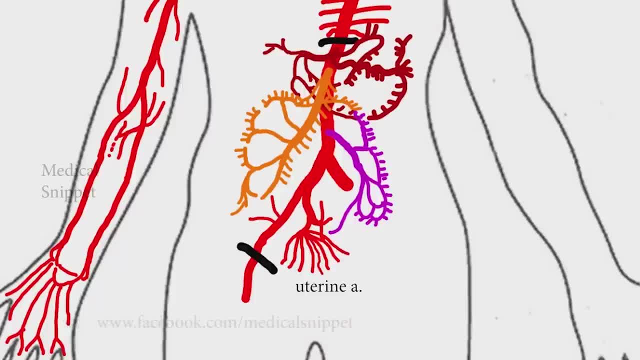 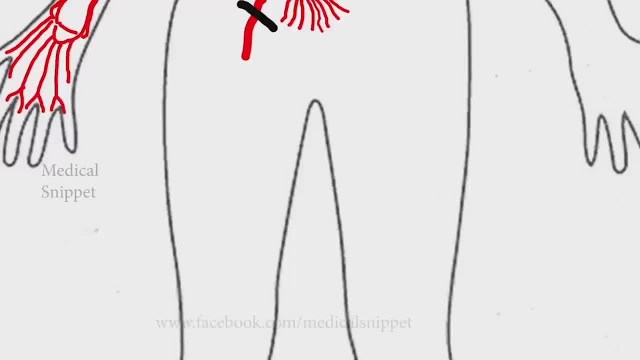 In females there is additional branch called uterine artery. The common femoral artery is a continuation of the external iliac artery. It gives rise to superficial epigastric artery, superficial and deep external pudental arteries and superficial circumflex iliac artery.